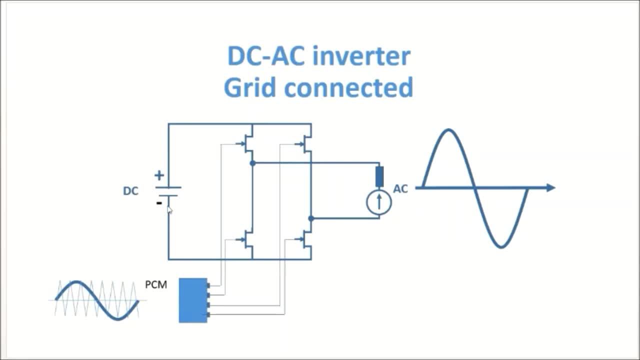 either pump electric energy stored in the battery to the grid or the other way around, utilize power of the grid to charge the battery. as i said earlier, the grid could either be a motor, a generator or whatever. so first we talk about the grid voltage and the second thing, which is important, it's the control signal. for a better understanding, 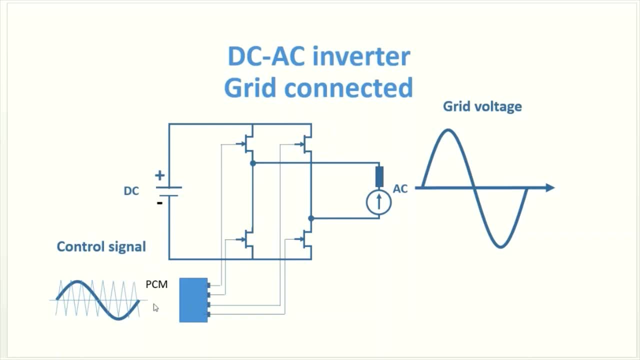 i shift the control signal under the load voltage signal or the grid voltage. so you have here the grid voltage signal and the control signal, which is just the grid voltage and the control signal generated inside the controller. so grid voltage signal, control signal. the next thing is that i make sure that both of these 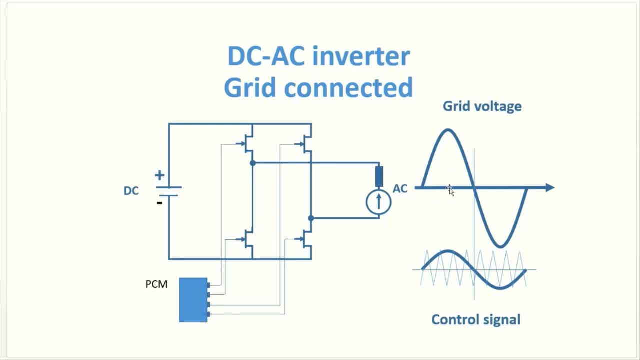 signals are absolutely in sync. that means they are exactly in phase. so this control signal is now in phase with the grid voltage signal. as long as the grid voltage and the control signal voltage are in sync, there is no real power exchange between the battery and the load. the only thing which 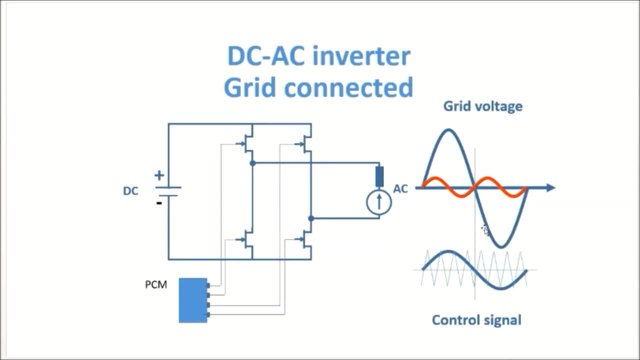 is exchanged is reactive power. it is exchanged at double the fundamental system frequency. in this case it could be 50 hertz or 60 hertz, for example, in us. otherwise, at the moment, no power exchange. by the way, the power exchange, of course, is the red curve. now we want to start to push. 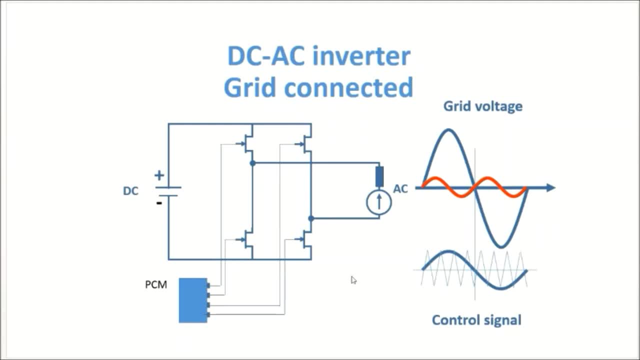 power from the battery to the network. in order to do so, we will start to to give the control signal a certain phase shift compared to the grid voltage signal, meaning we start to give it the leading edge. then you can see how we give it a leading edge, so move it in this direction and, as a result, we see that the power 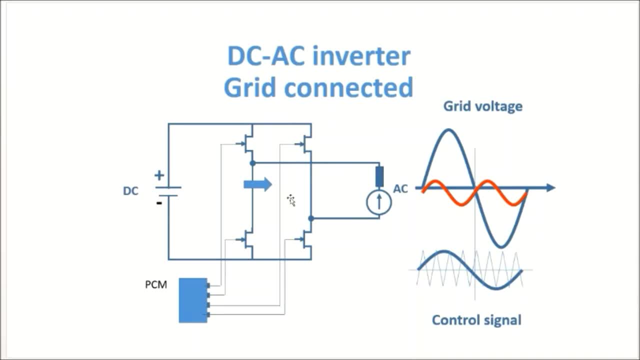 from the battery starts to be pushed into the grid, and we can even go further. you see, the power is increasing as long as we shift the signal and give it a leading edge. so the power is shifting, we get the maximum and all is in as a is a function of the leading edge of the control signal. 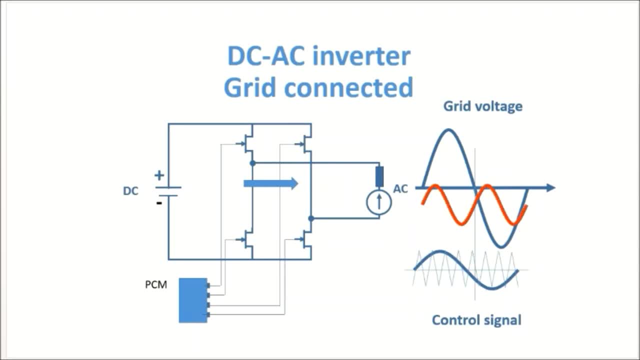 versus the grid voltage signal. we take back the leading edge a little bit and then the power goes back. it goes back to zero, where we have again reactive power, as at the beginning, and then we start to pump power from the grid back to the battery and, as a result, we can now see that 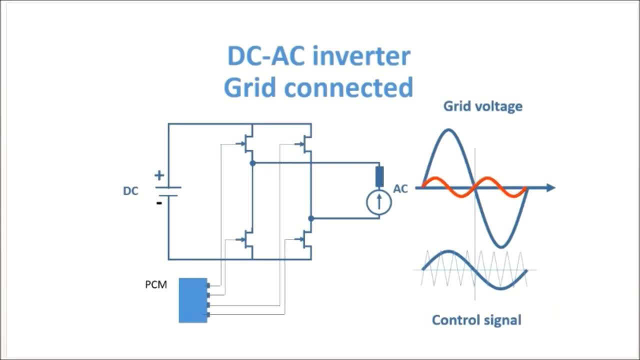 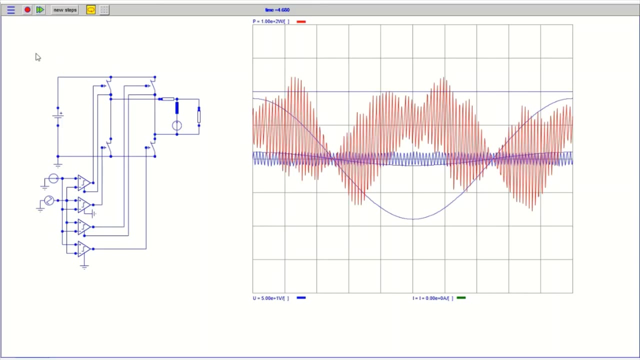 this is moving back and forth as a function of the lead of the control signal versus the grid or motor or whatever other signal we have. well, let's now have a look at my little simulator. you can access the simulator on wwwecspch. now you see that i have replaced this passive resistor from the inverter. lesson: 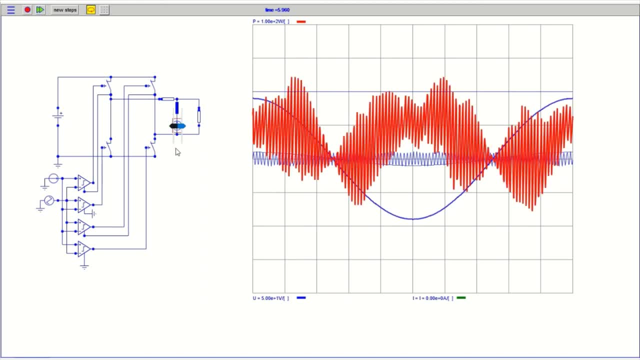 by an active component, in this case it's a. it could be a motor, it could be a grid connection, it could be a generator or whatever. what you see here now is that the signal from the load- the blue curve here- is in perfect sync with the signal generator. 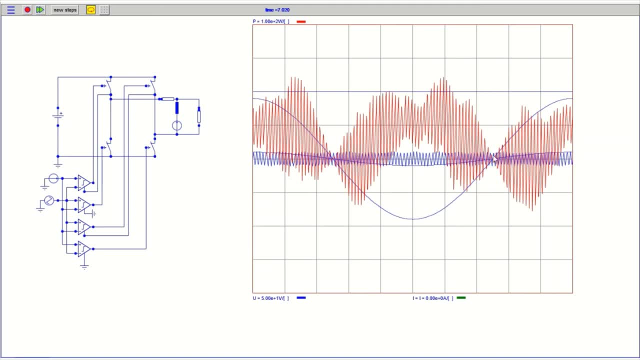 from my PCM controller so they have the zero crossing exactly at the same point. so it's in perfect in phase and therefore the power flow from the battery to the load is limited. the mess, what we see here, is because of the PCM modulation. in real life this frequency would be much higher and then you would not see such a 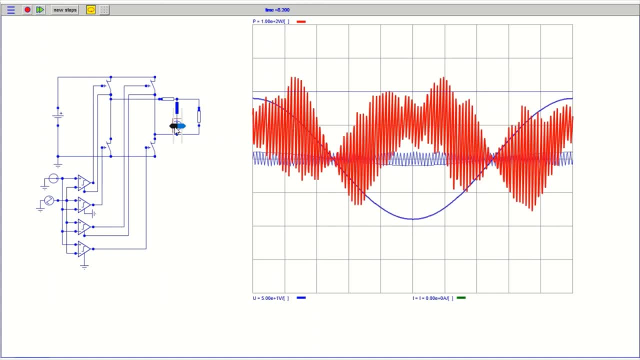 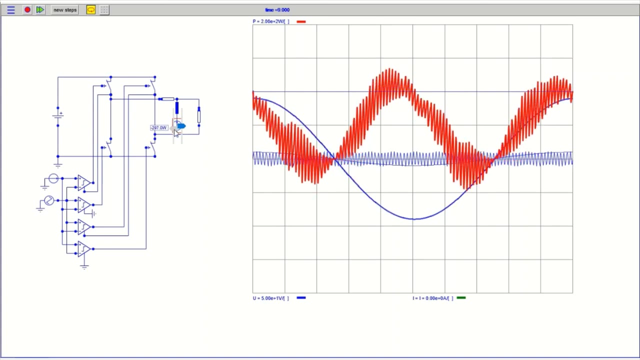 disturbance. now I have a motor here, for example, and I would now start to break the motor slightly. so I push power from the battery into the motor and you now see that the voltage signal of the load- here this is the load signal from the load- starts to phase shift, compared to the signal from the signal generator. 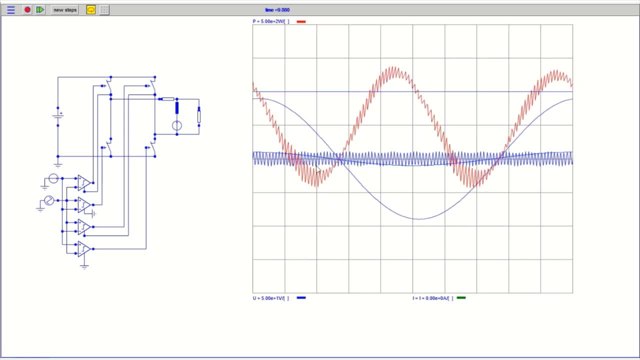 and therefore you start now to pump power. this is the red curve: power from the source to the load. we can continue and even go for more power. so what? in a, in a, In a car, now an electric car. this would mean that I would push the car, so I would.